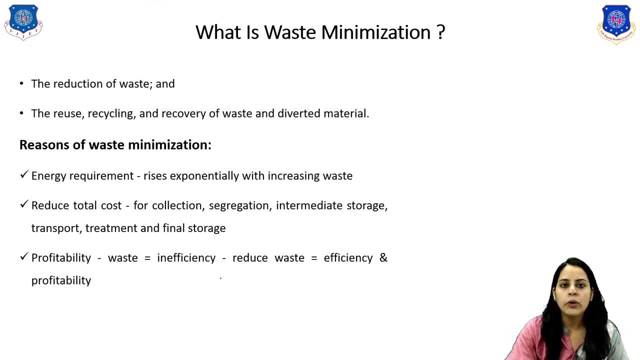 Okay, in previous lecture we have discussed about the Environmental Protection Act and Rule 1986 and the Factory Act, which is 1948.. Okay, now in this lecture we will discuss the What is a waste minimization? Okay, so, first of all, what is waste minimization? 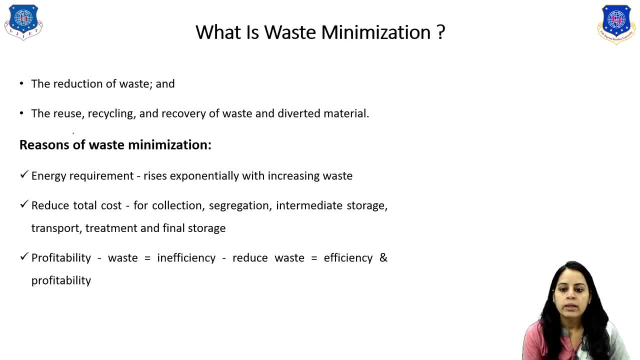 So it means that the reduction of the waste and reuse, recycling and recovering of the waste and diverted material. Okay, so the reason for the waste minimization, which is the first, which is it is an energy requirement, that it reduce the total cost and it is a profitability. 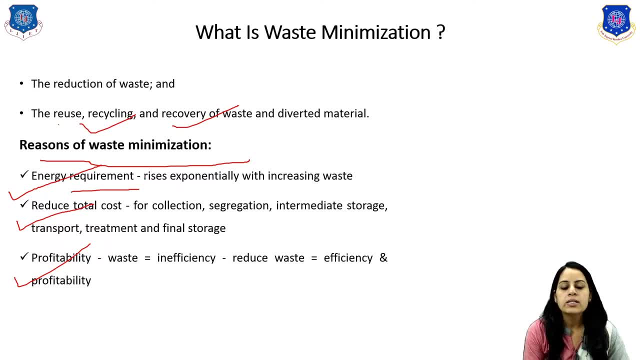 Right. so the energy requirement. it means that, Spontaneously with increasing waste, that it is a reduced total cost. it means that for collection, then segregation, intermediate storage, then transport and treatment and the final resource, Right, profitability. it means that in inefficiency minus the reduced waste, it means that efficiency and profitability 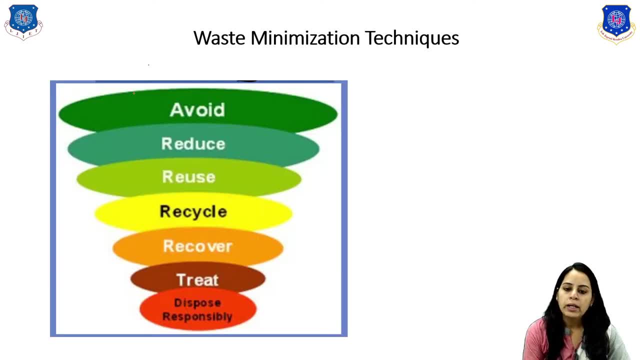 Okay, now the waste minimization technique. it means that the first step, which is avoid, avoid the waste, waste, reduce the waste, reuse of the waste, recycle of the waste, then recover of the waste, then treatment of the waste and the last one, which is the disposal responsibility. 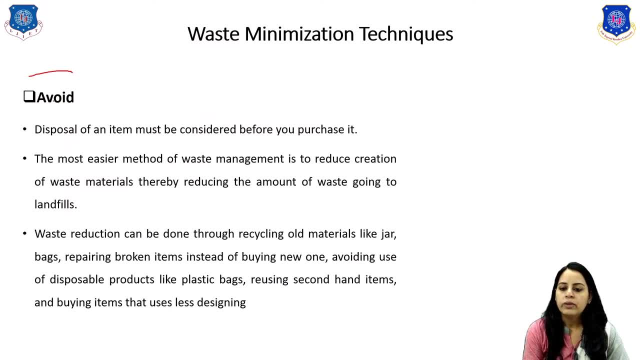 of the waste. Now we will start with the first one, which is avoid So the disposal of an item that must be considered before you purchase it. So the most easier method of the waste management is to reduce creation of the waste material, thereby reducing the amount of waste. 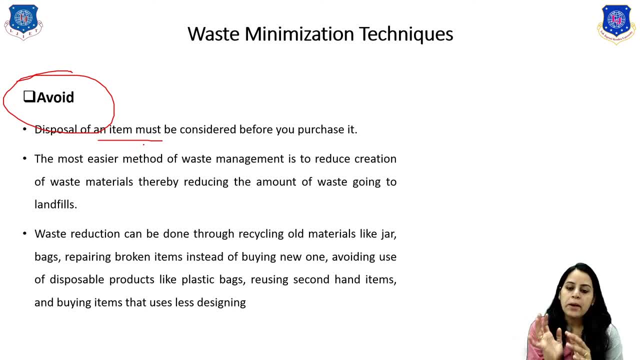 which is going to landfill. So the waste reduction, it can be done through the recycling of the old material, like a jar bag, repairing broken items then instead of buying a new one, avoiding the use of disposable product like a plastic bag, then reusing the second hand items then. 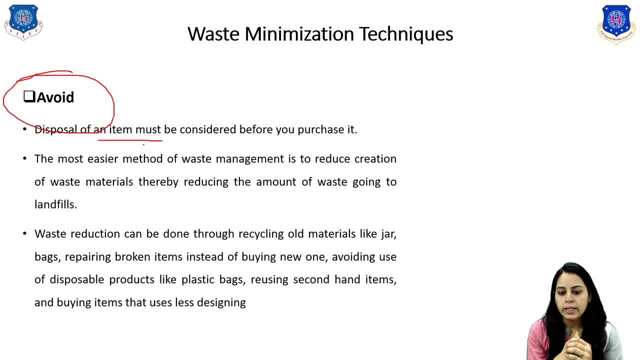 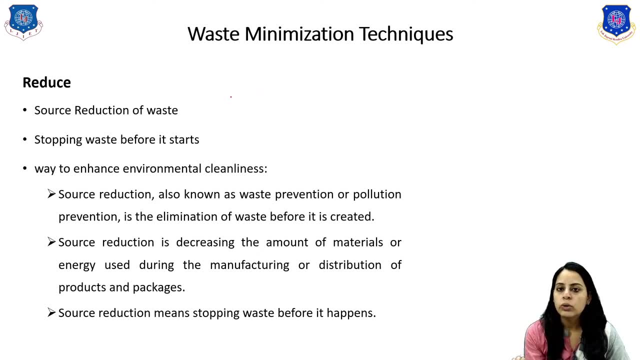 buying an item that is not used, So that useless design. it means that avoid The next one, which is the reduce. it means that reduction in the source of the waste, So the source reduction of the waste, then stopping the waste before it is stuck, So the way to enhance the environmental cleanliness. 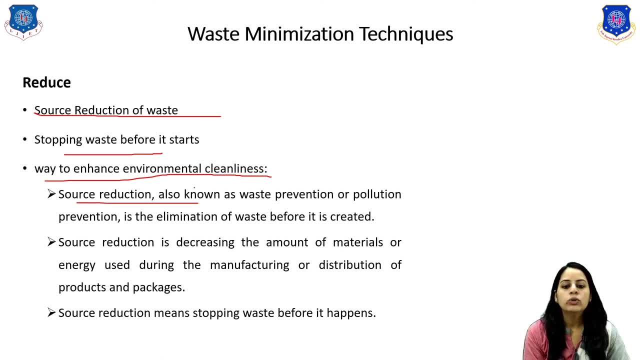 the first one, which is the source reduction, also known as a waste prevention or a pollution prevention, is the elimination of waste before it is created. So the source reduction is decreasing the amount of material or energy used during the manufacturing or distribution of product and the packages. The source reduction means stopping the waste before it happens. 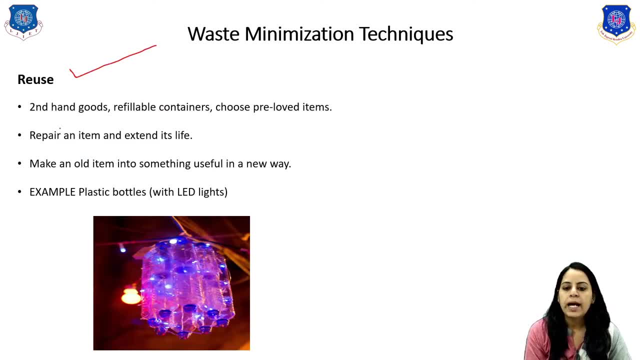 The next one, which is the reuse. it means that it is a second hand goods, then refillable container, then choose a pre love items. So the repair an item and extend its life, begin old item into the something useful in a new way. Here you can see that the example are: 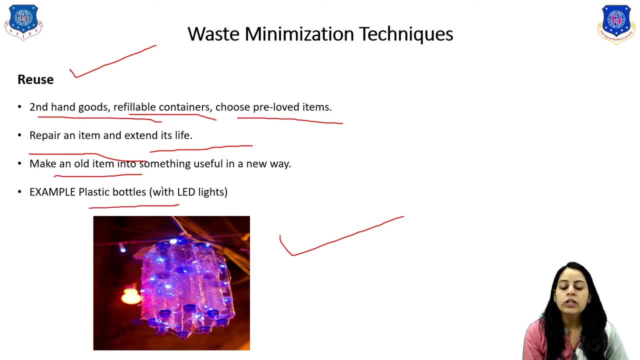 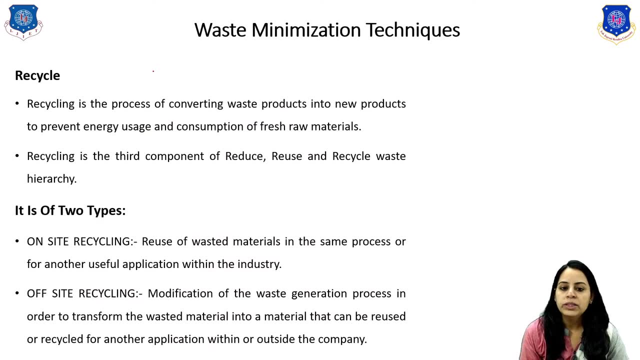 given the example, which is plastic bottle, which is reusable with the LED lights, right. So here the picture. you can see that Now. next one, which is the recycle. okay, So the recycling is the process of converting the waste into the new product. It means that 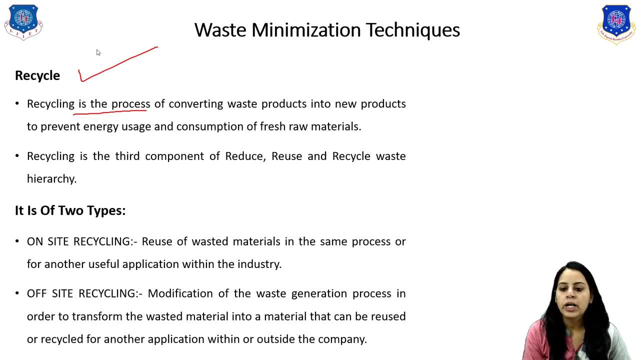 existing one which is replaced with the new one to prevent the annual waste. So recycling is the process of converting the waste into the new one to prevent the energy uses and consumption of the fresh raw materials. okay, It is a third component of the reuse: reuse. 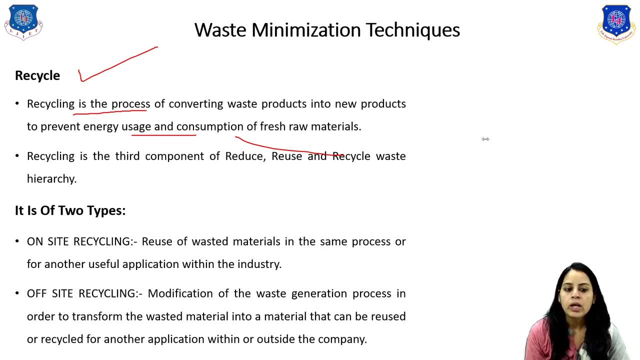 and the reduce, reuse and recycle waste hierarchy. So the idea behind the recycling is to reduce the energy uses and reduce the volume of the landfill, reduce the air and water pollution, then reduce the greenhouse gas emission and the preserve the natural resource for the. 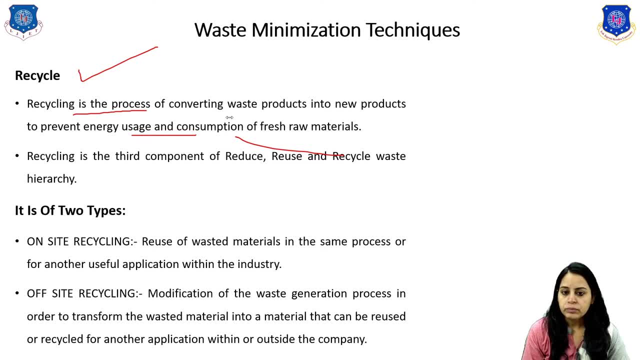 future. right Now, the recycling. it has the two types: the first one which is the on-site recycling, and the second one which is the off-site recycling, So the reuse of the wasted material in the same process or for the useful, another useful application within the industry. 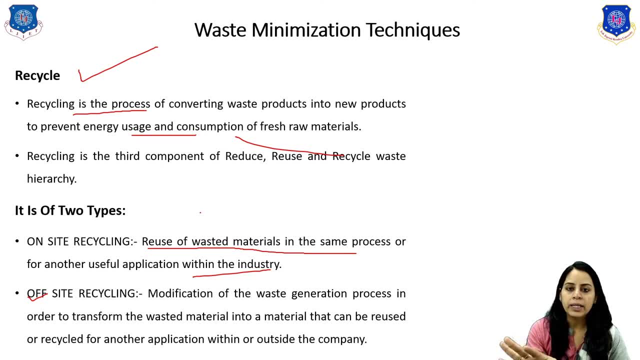 It means that on-site recycling- right, Because the material or the waste are useful in the same industry, right. Okay then off-site recycling: it means that modification of waste generation process in order to transform the wasted material into the material that can be reused or recycled for another application within or outside the companies, right This? 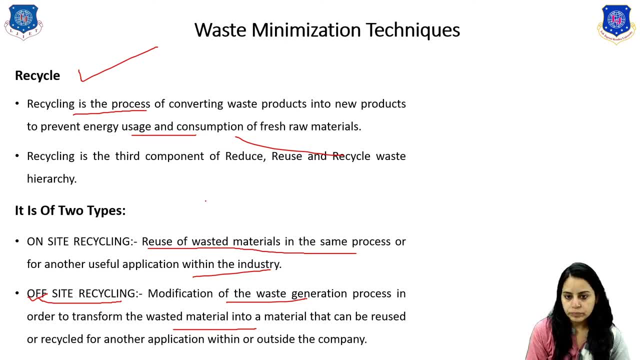 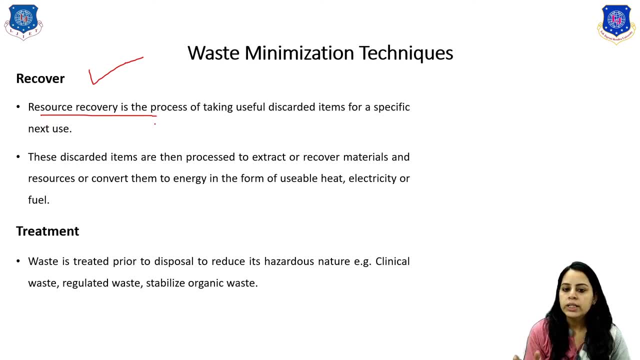 is a modification of the waste right. Now the next one, which is the recover. okay, So the resource recovery is the process of taking a discarded item for a specific next use, right, So this discarded item are then proceed to extract or recover material and resource. 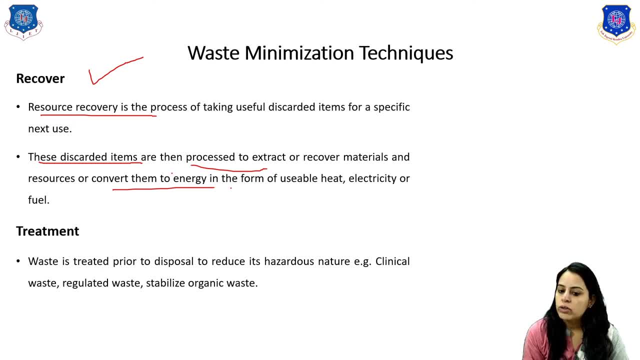 to convert them into them into to the energy in form of the usable, with electricity or so, recover. it means that resource to the waste, to the resource right, Recover. it means that the waste which is converted into the resources right, The next one, which is the treatment, 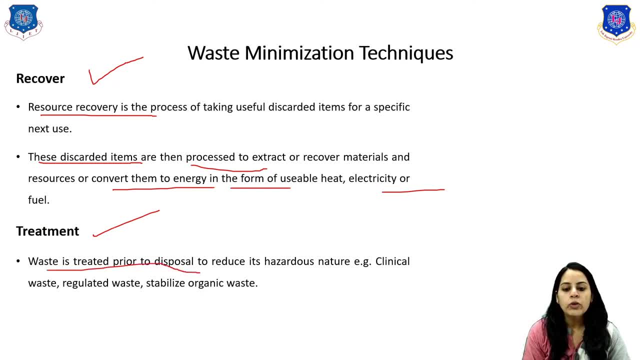 okay. So the waste is treated prior to dispose: disposal to reduce the hazardous nature: clinical waste, then regulated waste or stabilize the organic waste it means are treated. okay, There are lots of detailed treatment for the waste: physical treatment and chemical treatment. 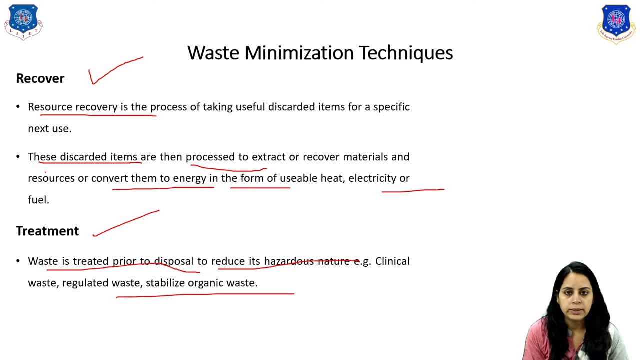 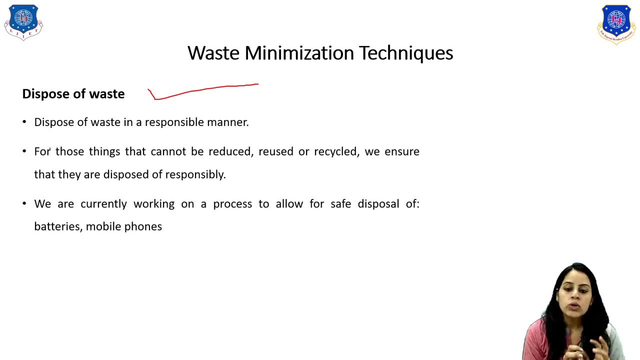 okay, Organic treatment and etc. Now the last one, which is the dispose of waste. it means that it is a for those thing that cannot be reduced, reuse or recycle, So we ensure that they are dispose of the responsibility right. So we are currently working on a process to allow for a safe disposal. 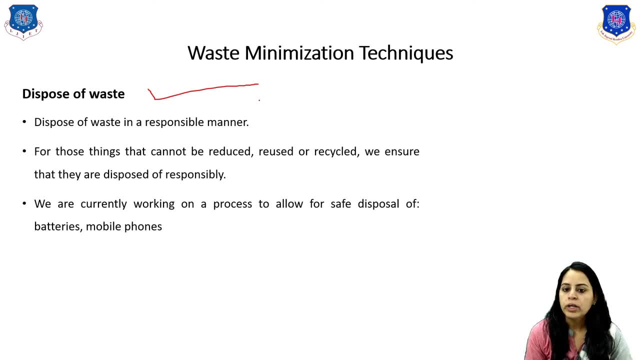 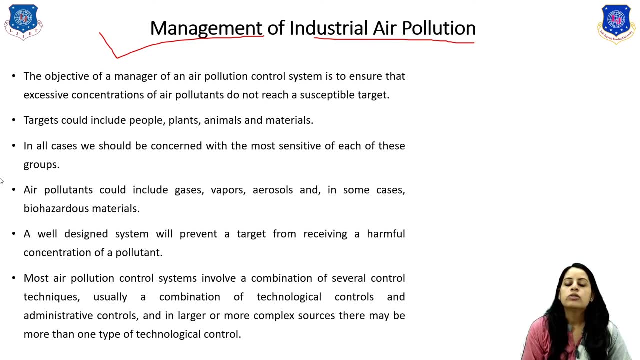 of the batteries and mobile phones and etc. okay, Now the next one, which is the management of the industrial air pollution. okay, So this topic is the management of the industrial air pollution, which is the industrial air pollution management system. So, the first one, which is the objective, okay, So, which is an air pollution manager, of the non-pollution. 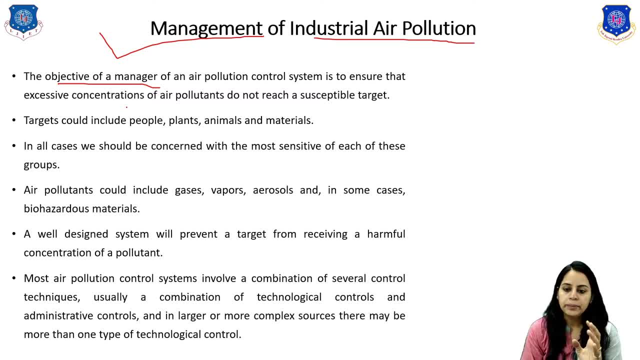 control system is to ensure that excessive concentration of air pollution, air pollutant, do not reach a susceptible target. okay, So the target could include the people, plant, animals and materials. okay, So in our case, we should concern with the most sensitive of each of this group, So the 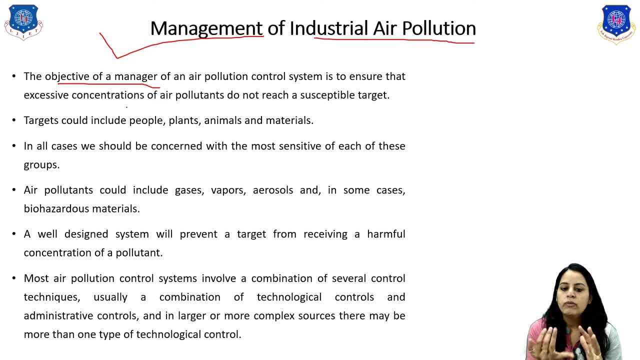 air pollutant could include the gases, vapour, aerosol and, in the some cases, biofasad material. okay, So a well-designed system will prevent the target from receiving a harmful concentration of the pollutant, and the most pollution control system involve the combination of the several: 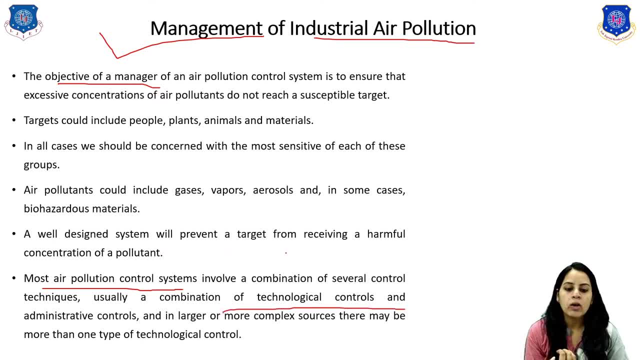 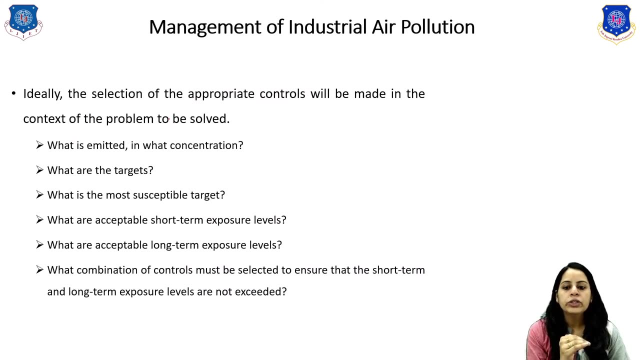 control technique, usually combination of technological and industrial technologies and the administrative control and the large or more complex sources. there may be more than one type of the technological control. okay, Now the ideally. the selection of the across side control will be made in the context of the problem to be solved. First of all, 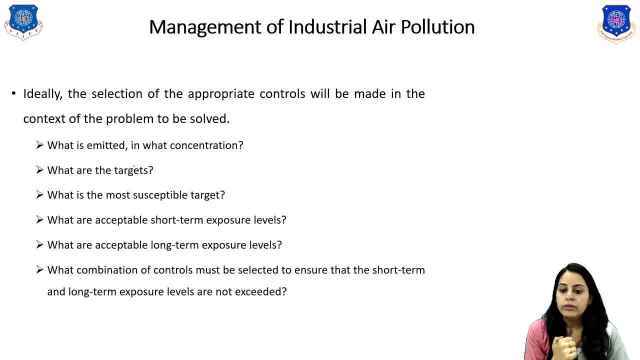 what is emitted in what concentration and what are the targets? what are the most susceptible target then? what are the acceptable short term exposure levels then? what are the acceptable long term exposure levels then? what combination of control must be selected to ensure that the short term and long term exposure level are not exceeded? okay, So these all are the 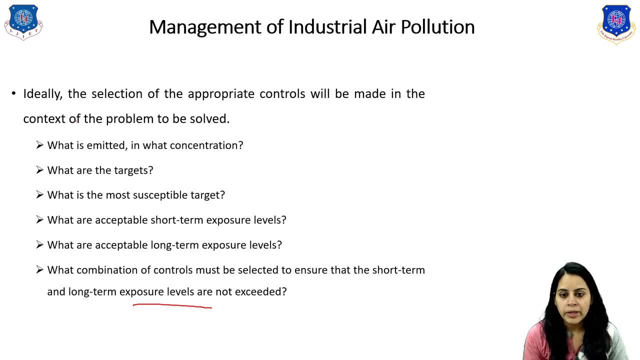 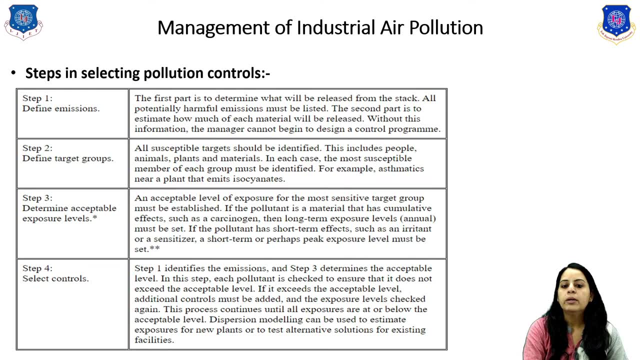 some question which is comes in our mind by the at the management level right Now. the next one, which is the steps in selecting policy and control. The first one, which is the define ambition. it means that this is the first part to determine what will be released. 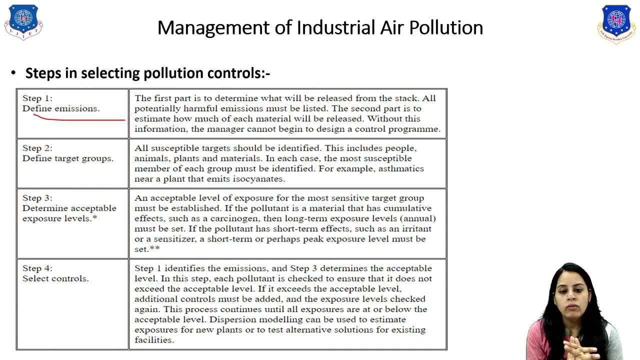 from this time. okay, All the potentially harmful ambition must be listed. The second part is to eliminate how much of each material will be reduced. So without this information, the manager cannot begin the design or control program right. Okay, now let us see the next. 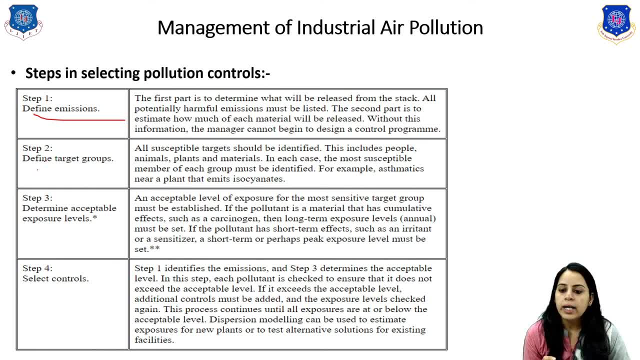 step, which is the define the target group. It means that all susceptible targets should be identified. After that, this includes the people, animal, plant and material. In each case, the most susceptible member of each group must be identified, For example, asthmatics. 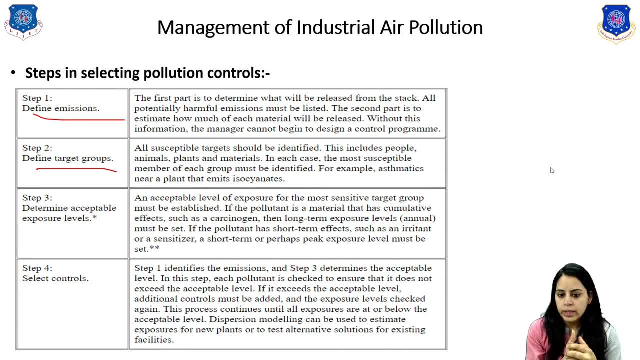 near a plant that have made up isodine right. Then step three: define the target group. Step three, which is determine the acceptable exposure level. It means that an acceptable level of the exposure for the most sensitive target group must be established If the pollutant 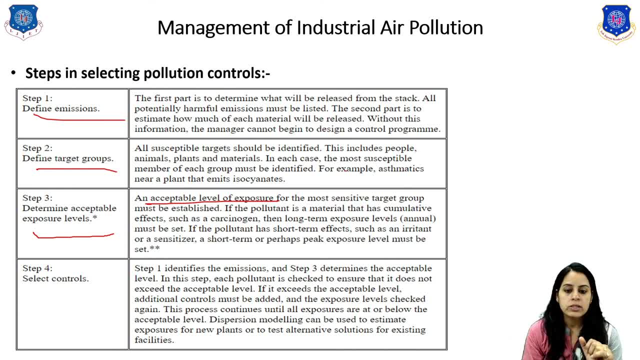 is a material that has cumulative effect, such as a carcinogen, then long term exposure level annual must be set okay. So if the pollutant has a short term effect, such as the irritant or a sensitizer or short term pollutant, then the target group must be established right. 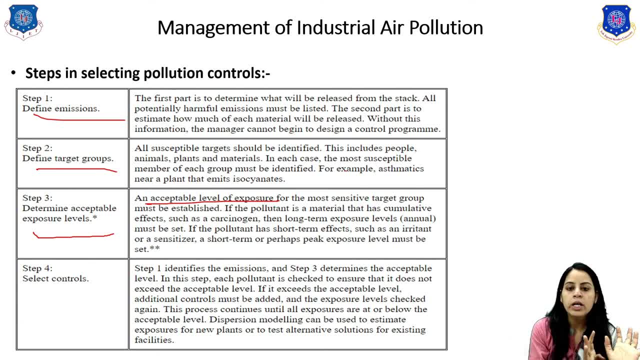 If the pollutant has a short term effect, such as permanent exposure level during the environment, then the target group must be established. So in this case, the target group is determined by determining the acceptable level of the exposure. Okay, And then step four: we just select the control technique. okay, So the in step one, identify the emission. 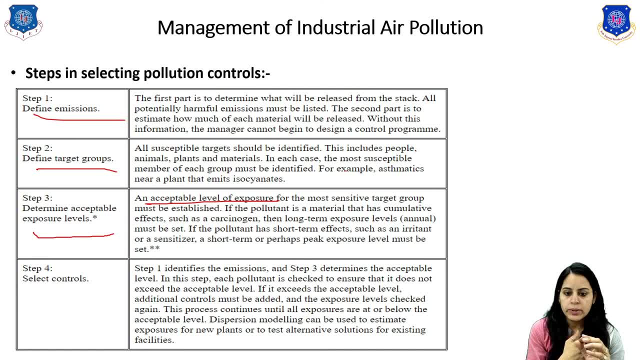 First we have to identify the emission and in step three we determine the acceptable level of the OK. So in this step, each pollutant is checked to ensure that it does not exceed the specific level. Okay, In this step each pollutant is checked to ensure that it does. 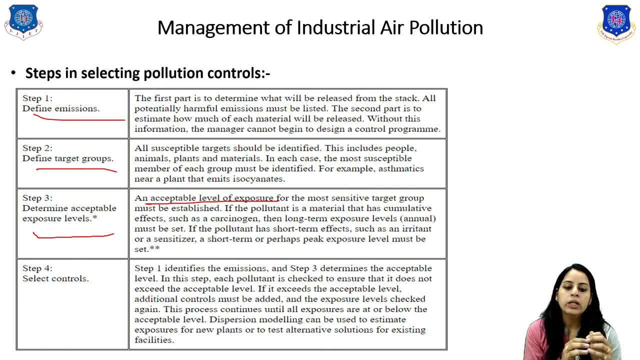 exceed the acceptable level, and if the it exceeds the acceptable level, so the additional control must be needed. okay, so the exposure level check again. this process continue until all the exposure are at or below the acceptable level. right, so the dispersion modeling can be used to estimate the. 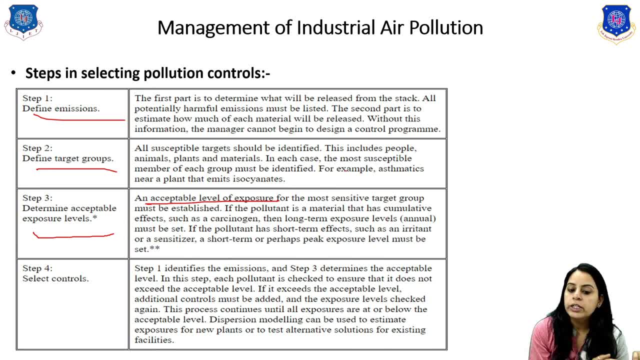 exposure for a new plant or a taste alternative solution for existing facilities, right? so this is the various steps in selecting the volunteer pollution control. the first one, which is the define: first of all, we define the application, right, uh, it means that to determine what will be released from this time, okay. then the second one, which is the define, the target group. it means 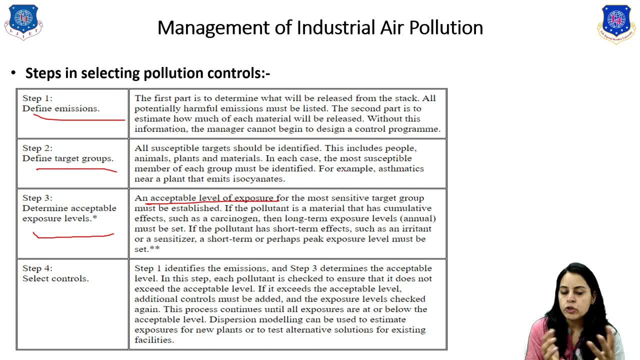 that, first of all, it should be target, should be the identity point, right. okay then step three. it means that determine the acceptable exposure level. it means that it is a less, a less exposure level than a short term or long term exposure level. right, and the last four. 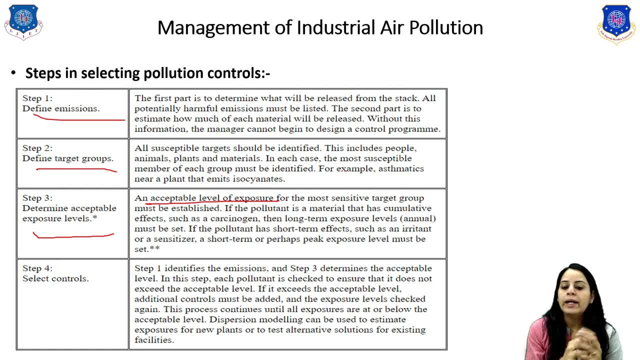 which is the select, the control right. for example, if we identify the emission, then determine the accepted level. so in the search that in such a time the pollutant is checked, we saw that it is not exactly acceptance level. if there are exceed the acceptance level, then we select the select, the another control for this particular pollutant. okay, so this is the.